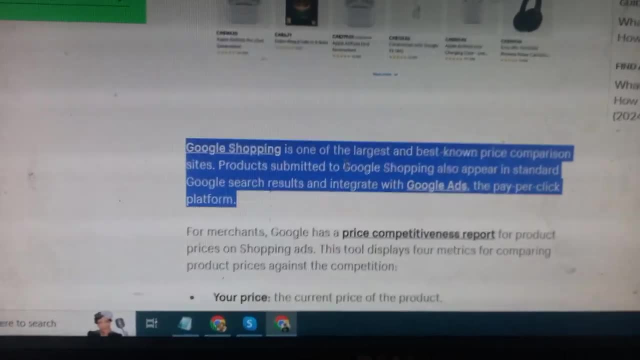 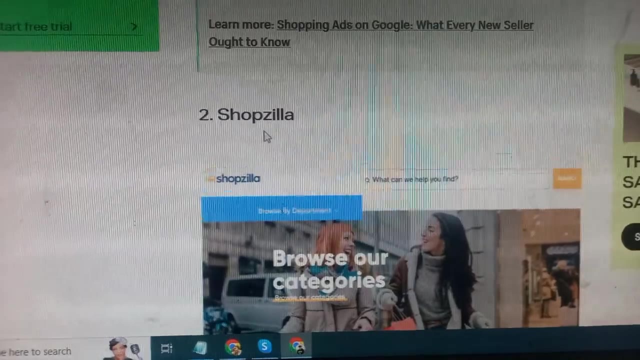 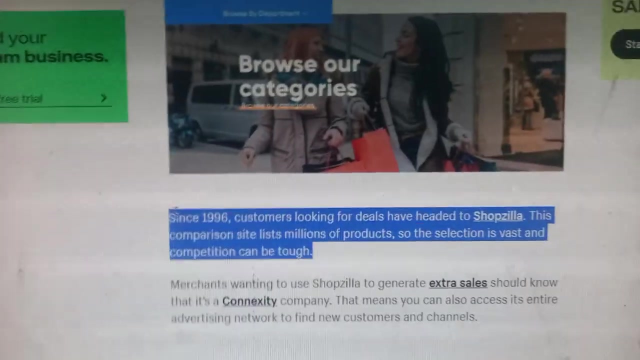 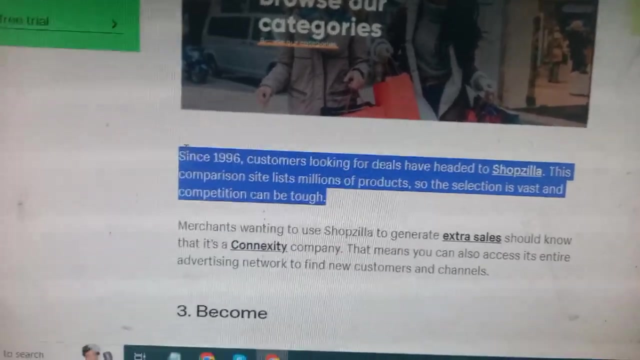 in standard Google search results and interrogate with Google ads. The pay-per-click platform Number two, Shopzilla. Since 1996, customers looking for deals have headed to Shopzilla. These comparison sites list millions of products, so the selection is vast and competition can be tough. 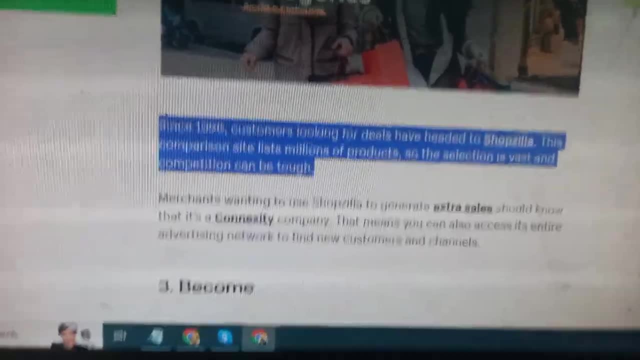 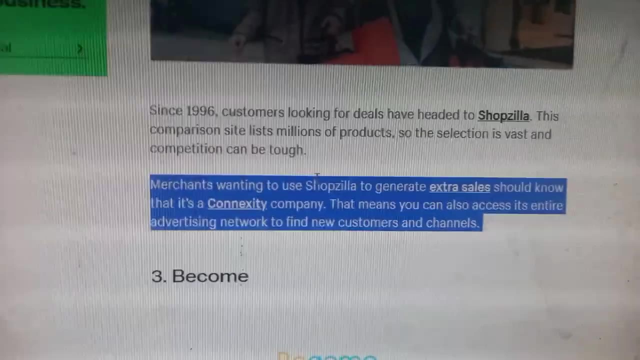 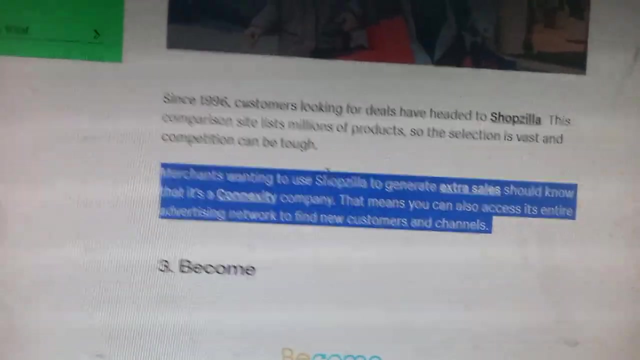 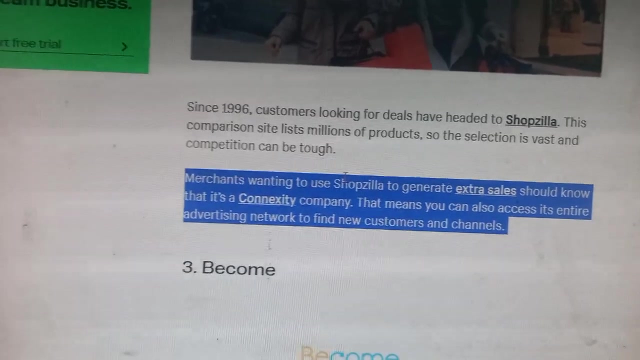 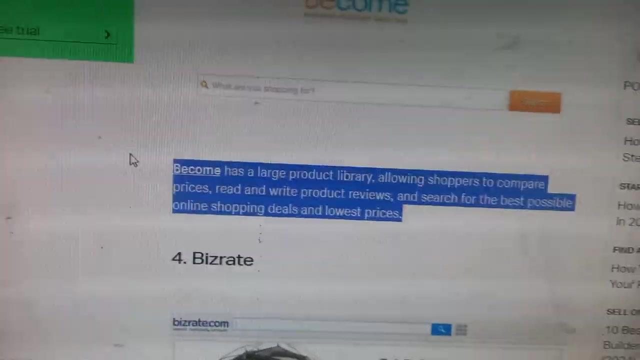 Merchants wanting to use Shopzilla to generate extra sales should know that it is a connectivity company. That means you can also access its entire advertising network to find new customers and channels. The search engine has a large product library allowing shoppers to compare prices. read: 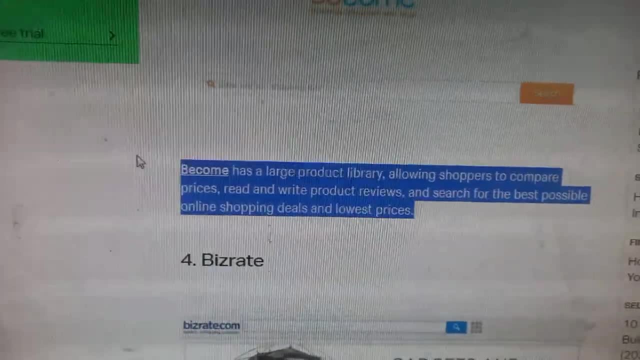 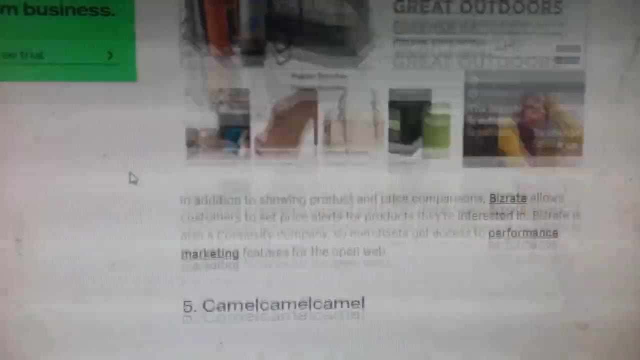 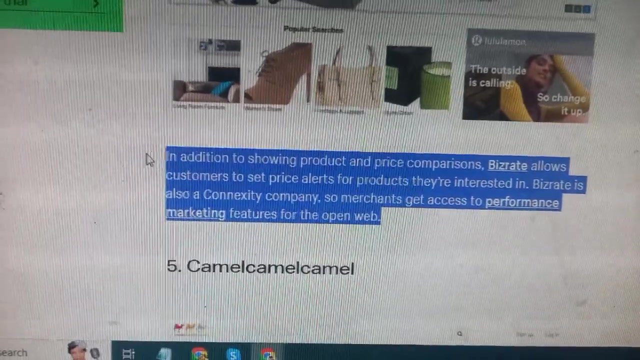 and write product reviews and search for the best possible online shopping deals. and lowest price bids rate. In addition to showing product and price comparisons, bids rate allows customers to set price alerts for products they are interested in. Number three: Google Shopping. Google Shopping is a new way to create a more authentic online. 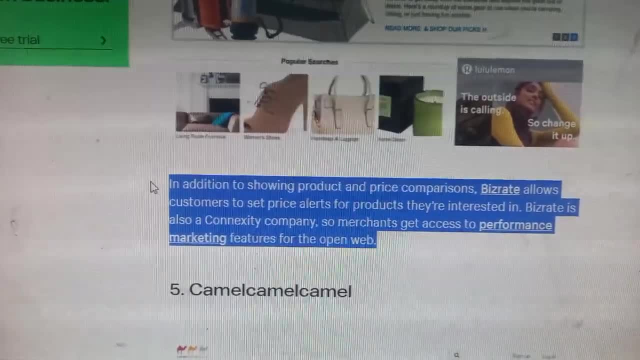 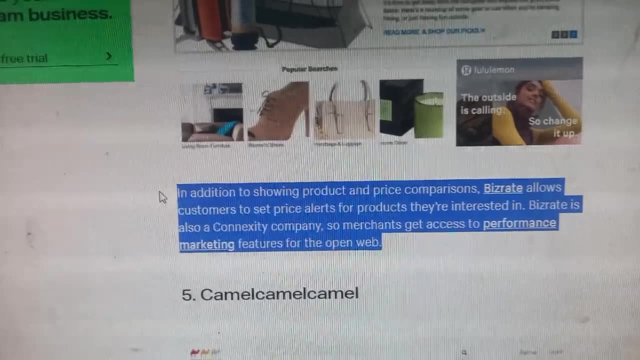 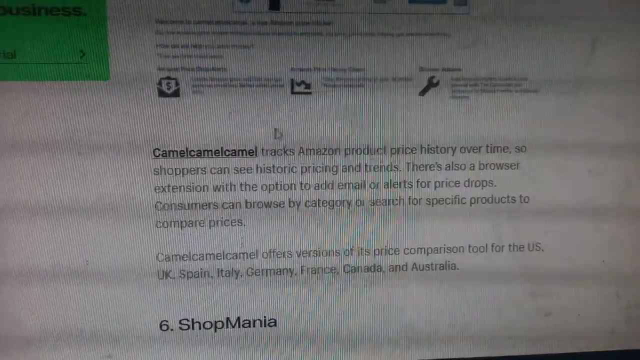 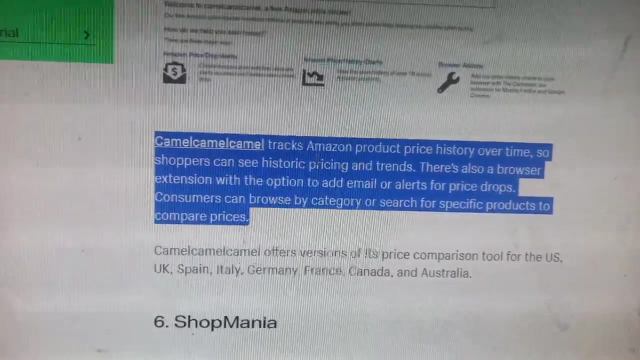 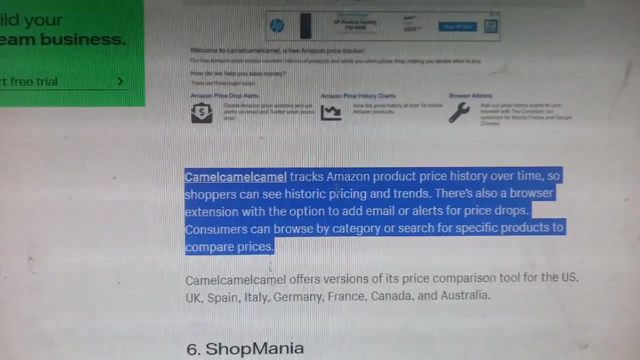 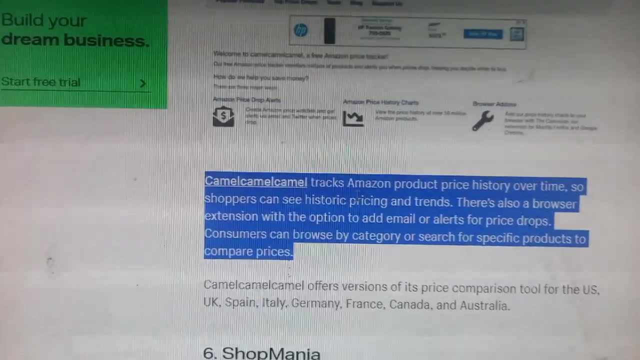 shopping experience. It is a platform where you can reach a large number of customers. These rates is also a connectivity company, So merchants get access to performance marketing features for open web. Camel Camel, Camel, Camel, Camel, Camel. Camel tracks Amazon's product price history over time so shoppers can see historic pricing and trends. There's also a browser extension with the option to add email or alerts for the price drops. 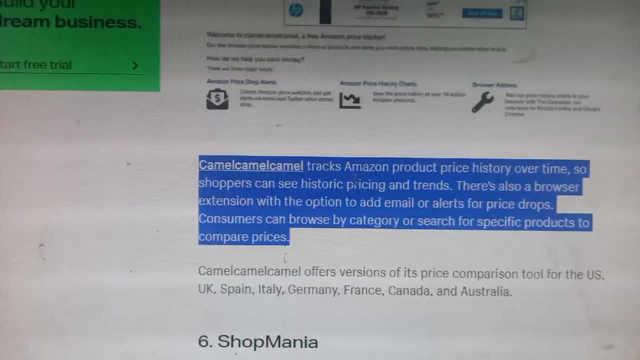 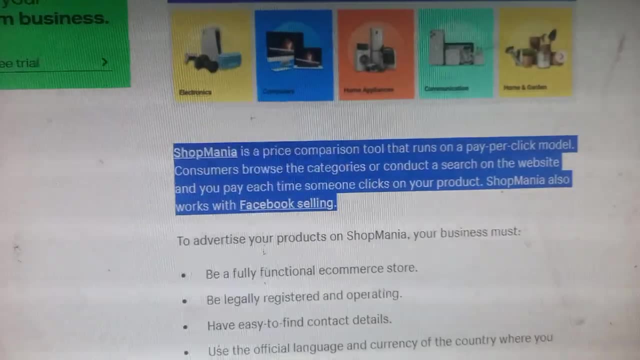 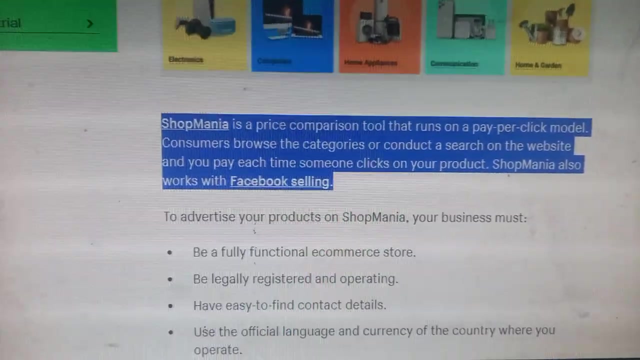 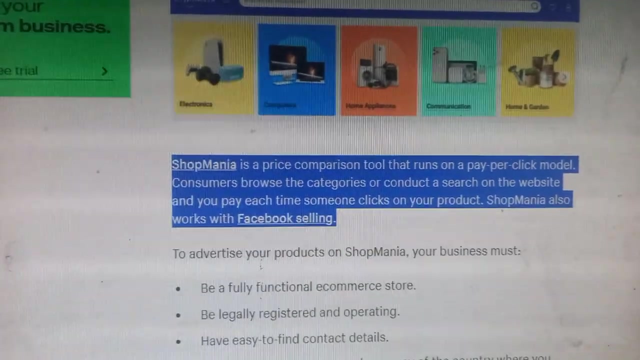 Consumers can browse by category Or search for specific products to compare prices. Shopmania. Shopmania is a price comparison tool that runs on a pay-per-click model. Consumers browse the categories or conduct a search on the website and you pay each time someone clicks on the product. Shopmania also works with Facebook selling.